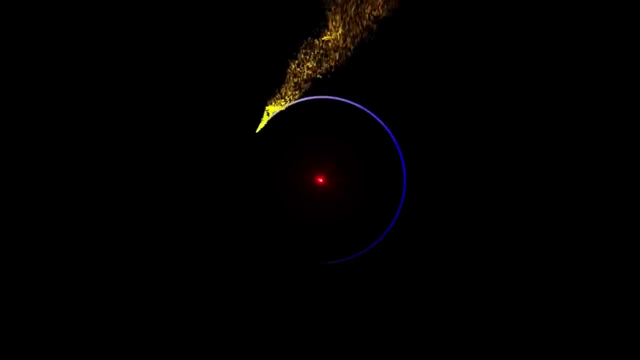 So here we go. Classical mechanics fail to describe how an electron could orbit an atom. An accelerating charge like that of an electron around a nucleus always creates electromagnetic radiation. according to Maxwell's classical equations, This means that the electron would constantly lose energy and eventually crash into the nucleus. Niels Bohr solved this problem by: 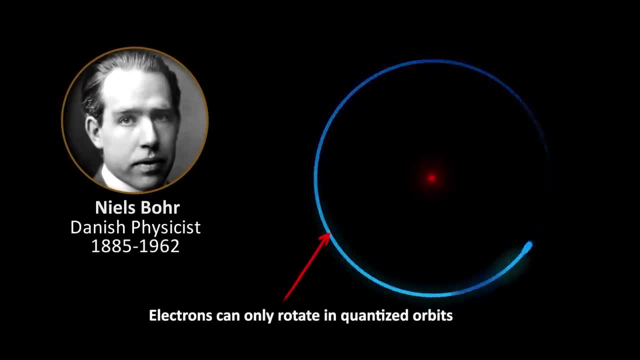 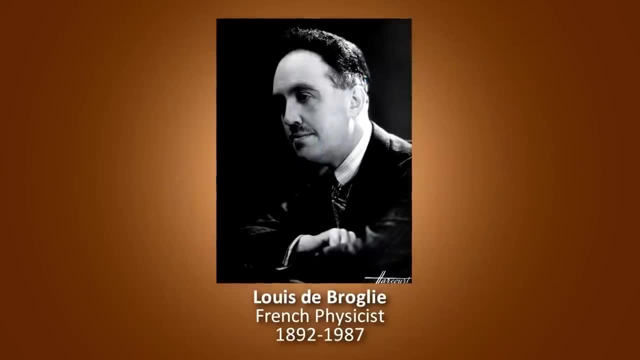 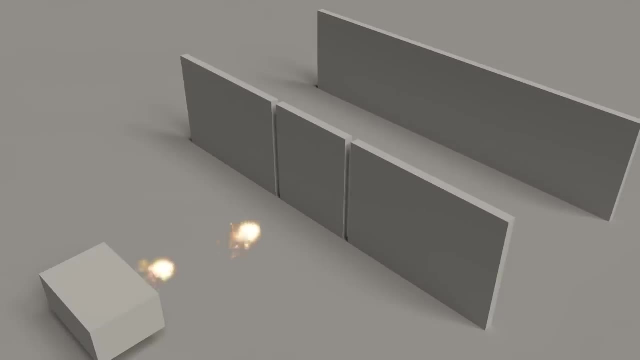 hypothesizing that electrons could exist without radiating energy if they rotated in quantized orbits proportional to Planck's constant. Louis de Broglie later showed that if such quantized orbits exist, then electrons must be waves. Astonishingly, experiments showed that not. 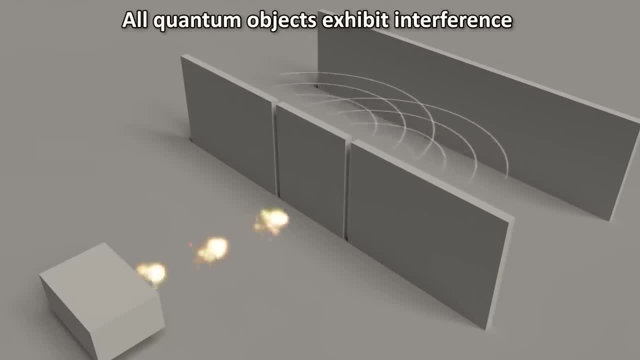 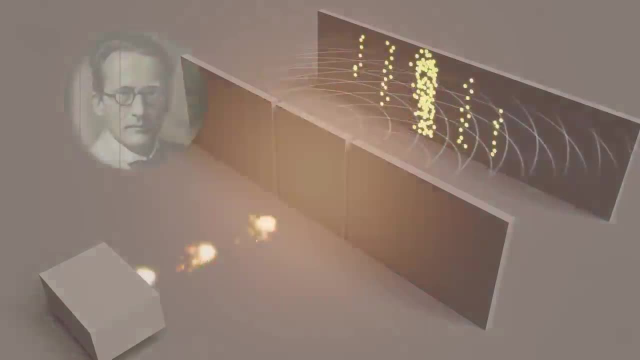 only electrons, but all quantum particles like photons and even atoms exhibit interference with no expression. This is not an easy task to do because of the many exceptions Implying. everything else must be waves too. Erwin Schrodinger developed an equation to explain this wave-like behavior. 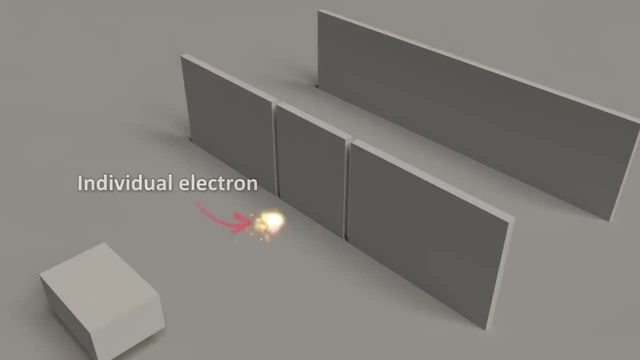 His equation describes how a wave evolves over time, But the problem is that whenever we detect these quantum objects, we detect them as particles, not as waves. This presents a conundrum. Experiments like the double slit experiment suggest waves, but detection appears to indicate particles. 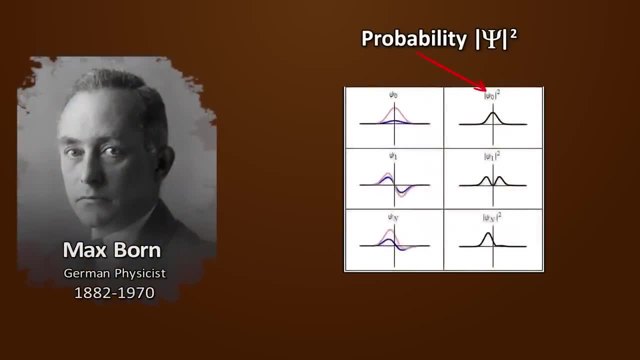 So Max Born came up with the idea that we should interpret the wave detections as waves and the expression to interpret the wave determined by the Schrodinger equation as a kind of probability. This allows a single quantum object to be described as a wave. So we've adopted a wave interpretation. 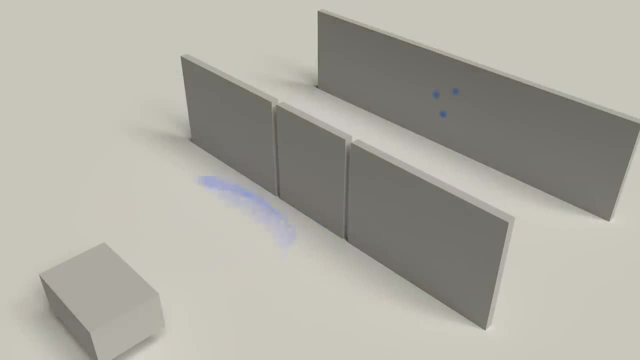 of a particle which evolves through time according to the Schrodinger equation And analogous to a classical wave. it does not have a distinct location. It has only a probability of being found at any particular location. This location can only be determined once we measure it. 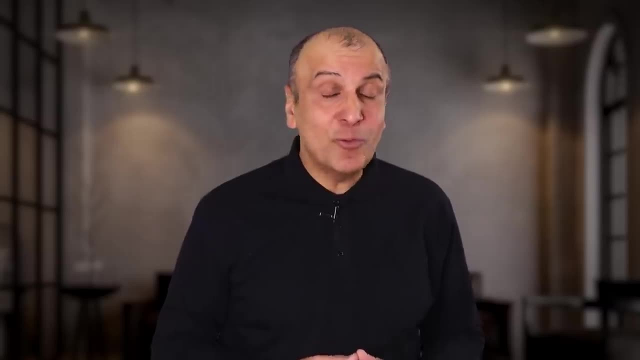 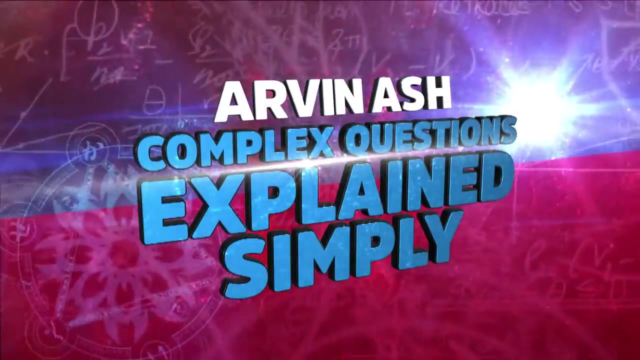 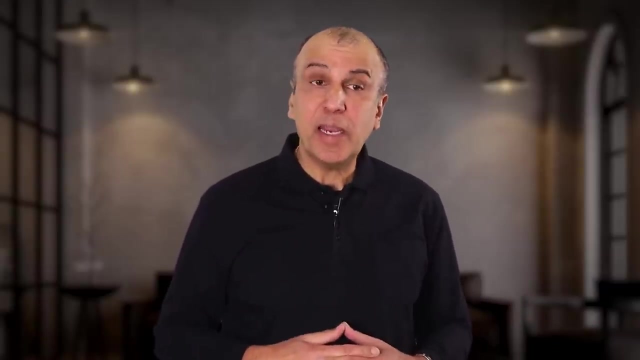 not in advance. So that's your 90 second summary. Now, if you are intrigued by this and want to understand this better and particularly ponder about what it all means, then stay tuned, because that's coming up right now. So, now that you know a little bit about the history of quantum mechanics, let me explain. 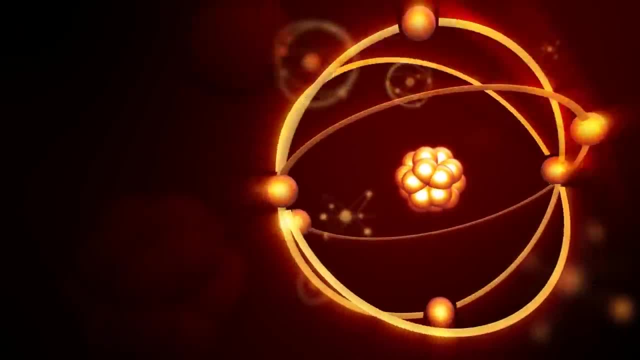 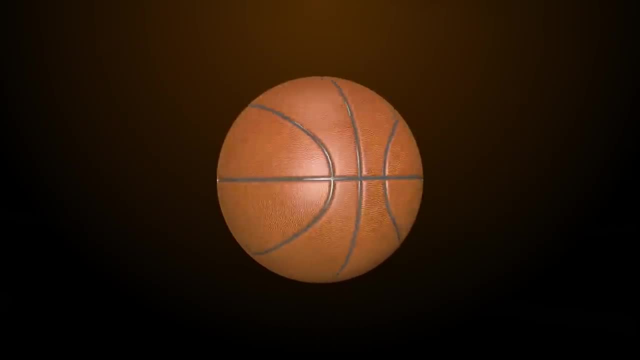 what the big deal is. It would be nice if we could just scale down everything we know about our macro world to the quantum world. For example, if the Newtonian mechanics of a basketball applied to electrons and atoms, there would be no problem. 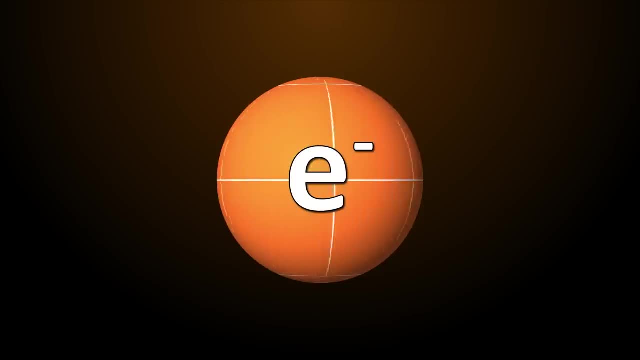 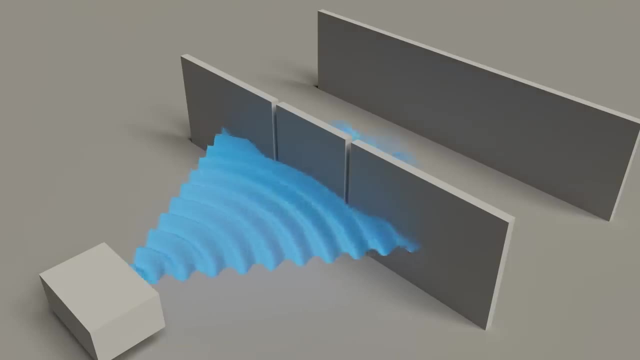 Everything would be intuitive and we could relate everything to our everyday experience. But the universe didn't make things so simple. for us, Quantum objects such as electrons, photons and atoms are not like little basketballs or tiny pieces of dust. They are like waves because they create interference patterns, like we see in the double slit experiment. 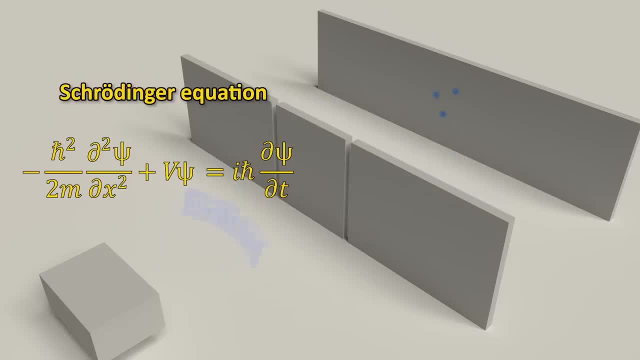 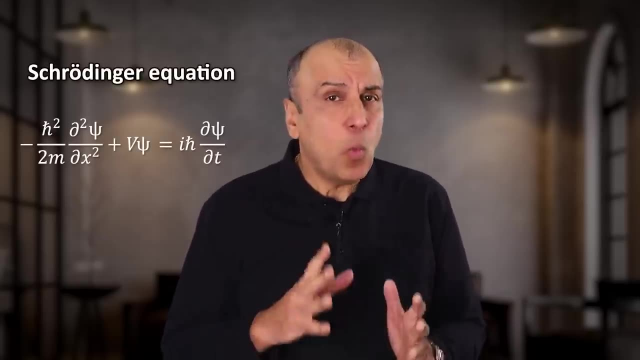 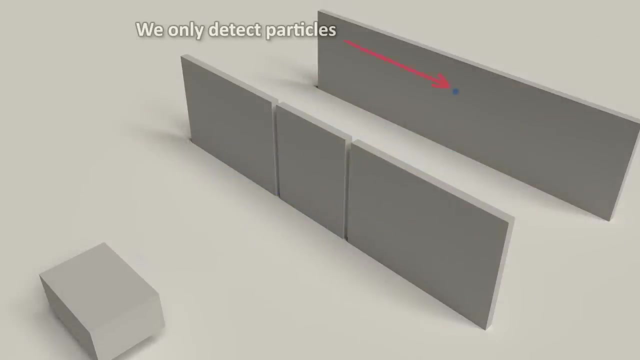 The Schrodinger equation was developed to explain how these waves evolve, And it's quite accurate. So if we have a rigorous mathematical model to describe these waves, what's the big deal, since we know how it works? The problem is that we only observe particles, or at least particle-like behavior, whenever. 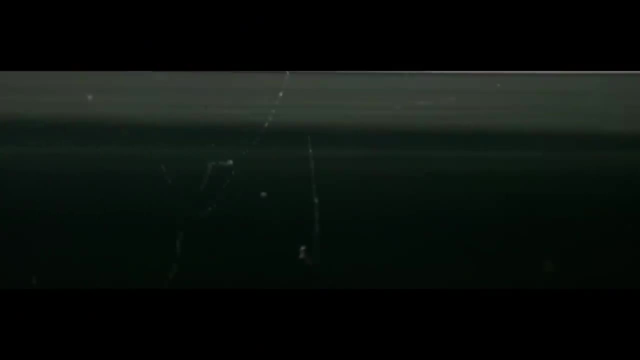 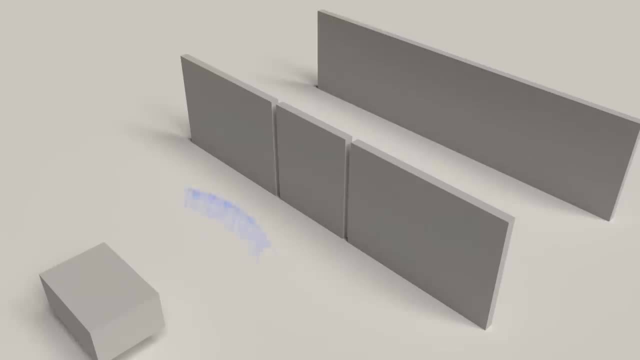 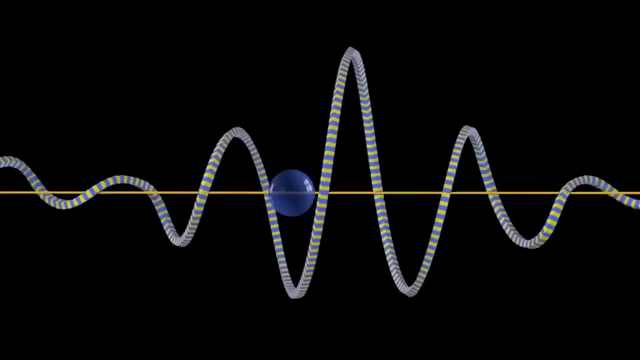 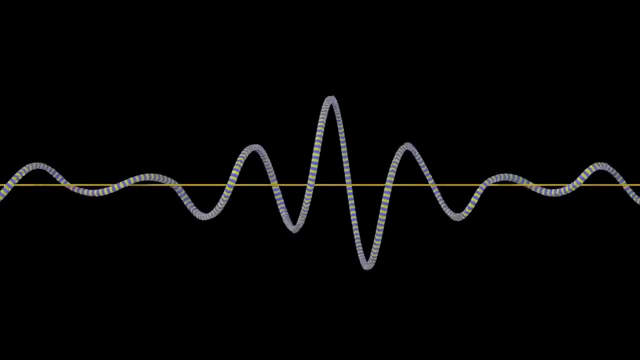 The subatomic objects seem to behave like particles, Not waves. So to incorporate this into our quantum mechanics theory, the concept of measurement was introduced. So you'll hear physicists say, at least in the most common interpretation of quantum mechanics, that whenever a measurement is made, the wave collapses and becomes a very 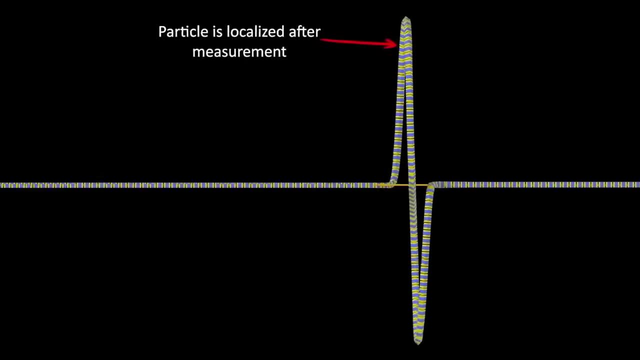 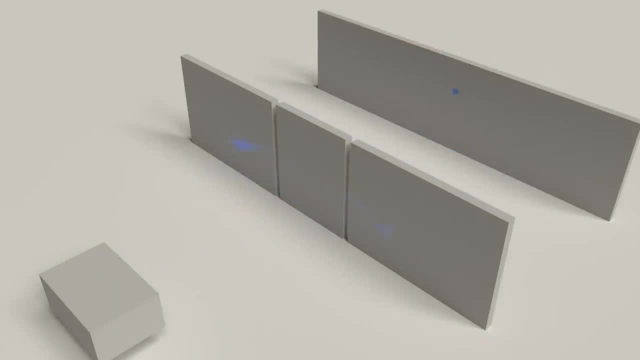 localized wave which effectively makes it look and behave like a particle. Measurement means an interaction, An interaction of the quantum object with some kind of particle. An interaction of the quantum object with some kind of particle. An interaction of the quantum object with some kind of particle. 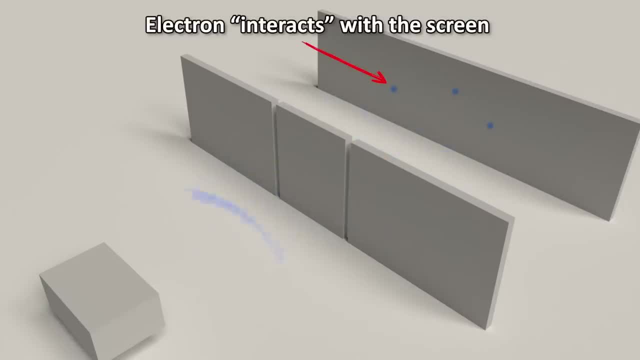 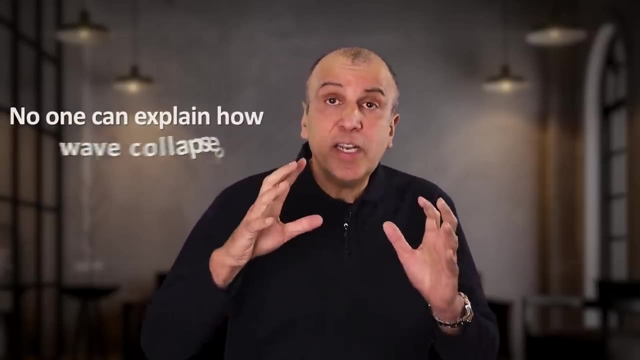 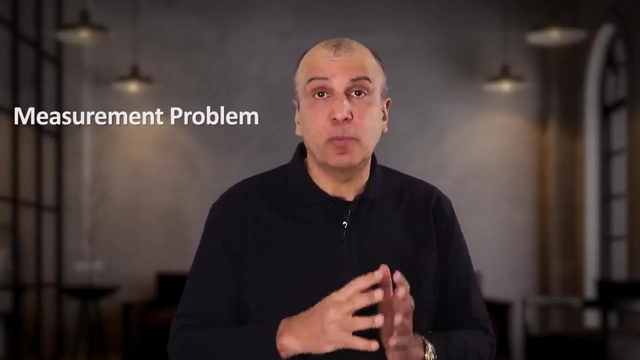 More specifically, an irreversible exchange of energy somewhere in the measurement process. This seems nice and clean, but there's a huge problem. No one can explain how or why this wave collapse occurs through measurement. This is called the measurement problem in quantum mechanics. 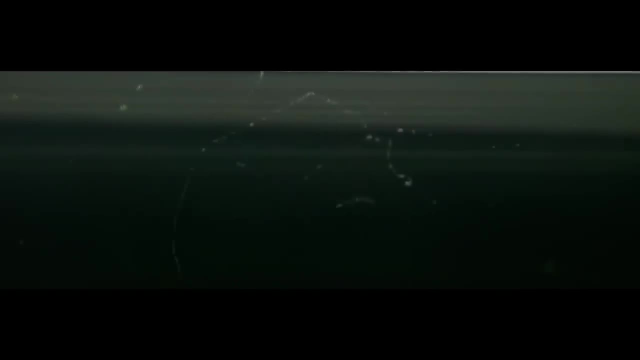 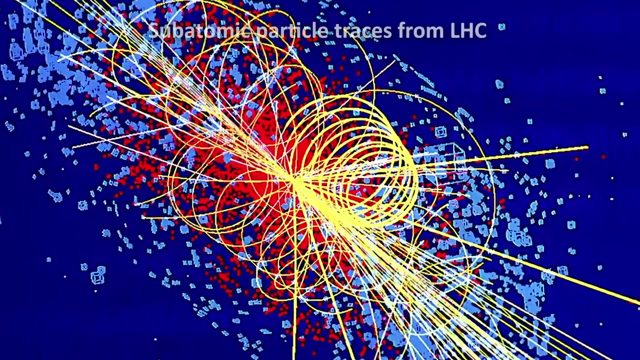 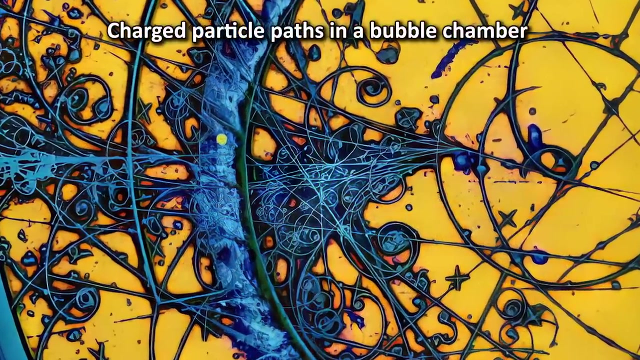 And since all our information comes from a measurement of some kind, we can never directly see or touch this quantum world. Everything we observe must go through this measuring process that seems to result in the conversion of quantum objects into particles, like the classical world we are familiar with. 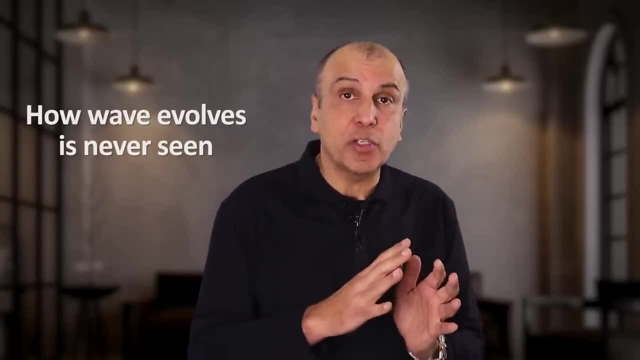 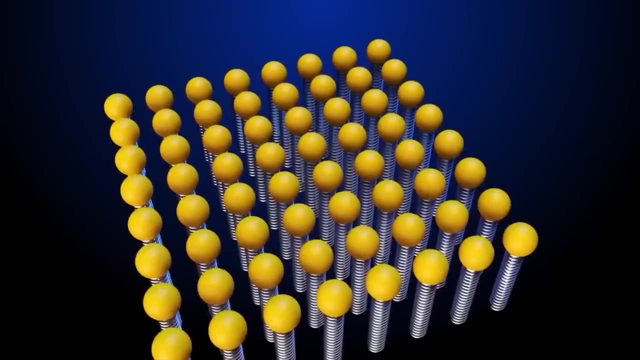 So how this wave evolves according to the Schrodinger equation, while it's highly accurate in making predictions, is never actually seen. Like I showed two videos ago, ultimately quantum theory boils down to a theory of interacting harmonic oscillators combined with a measurement postulate. 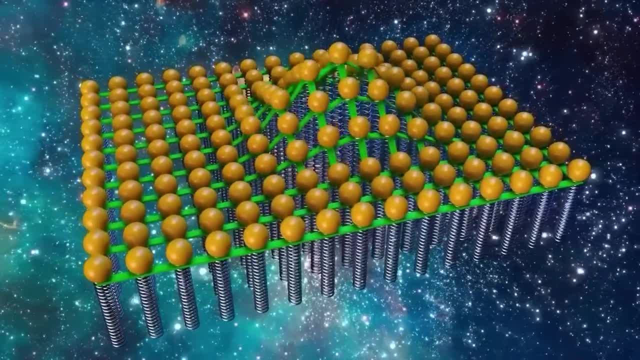 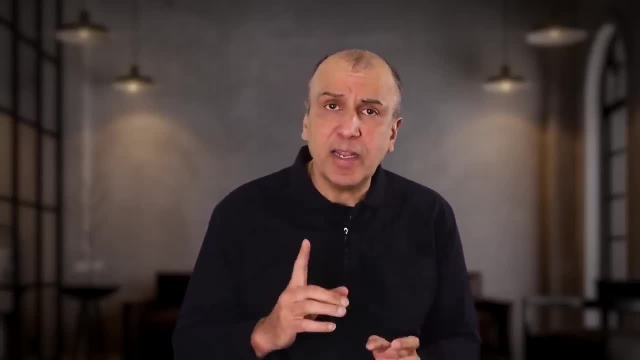 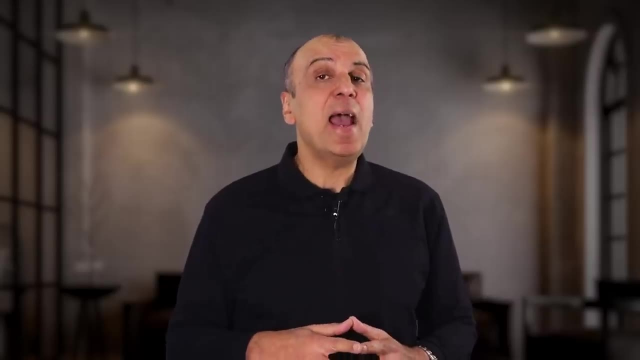 But no one can explain how the interactions of the harmonic oscillators are different than the interaction of the measurement device. If we really want to understand reality, this is a fundamental problem that we need to resolve Now. having said all this, let me add that not resolving the measurement problem has 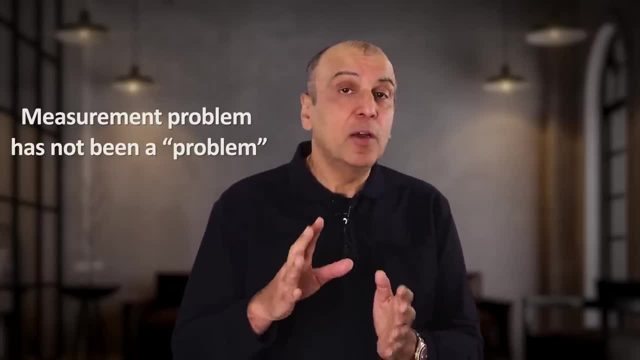 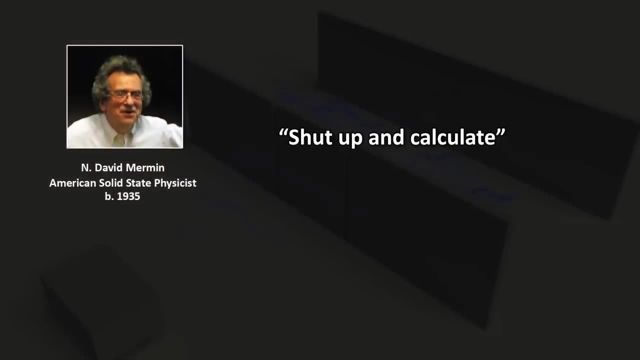 not prevented us from predicting and measuring outcomes from these equations. There is a philosophy called just shut up and calculate Meaning. don't worry about what's really going on. If the bottom line is that all our equations work and are highly accurate, that's all. 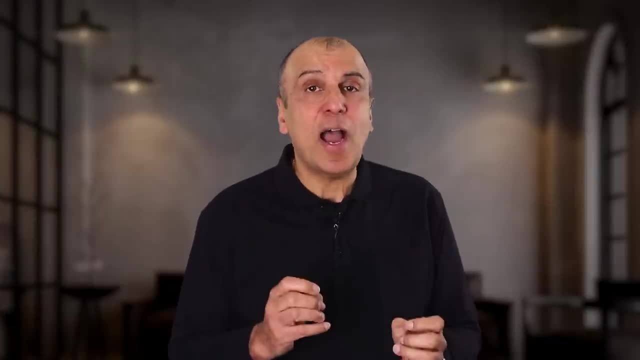 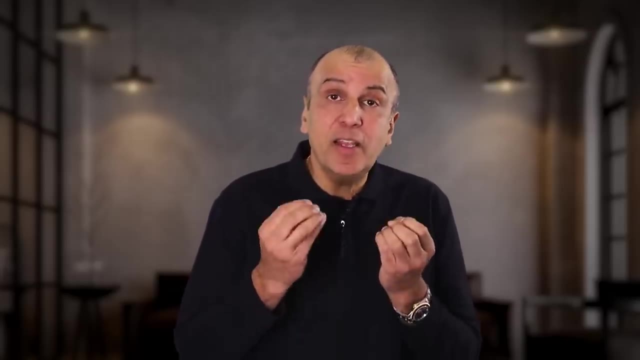 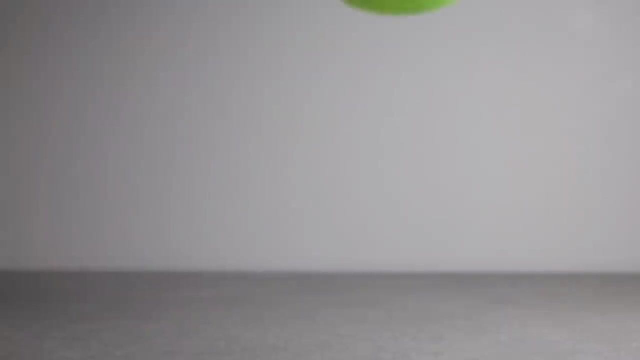 we should care about. I don't subscribe to this kind of thinking myself, because I think that the purpose of scientists, particularly physicists, is to explain the inner workings of the universe, not simply create equations that make predictions without a deep understanding. 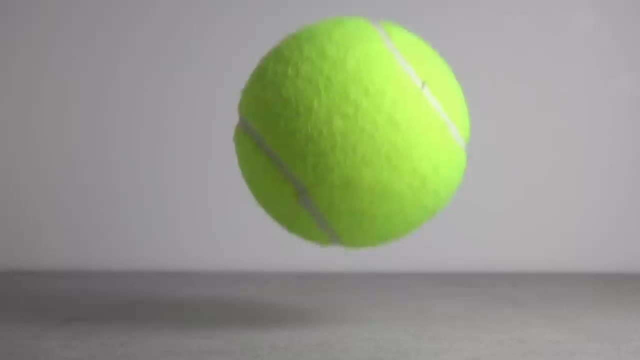 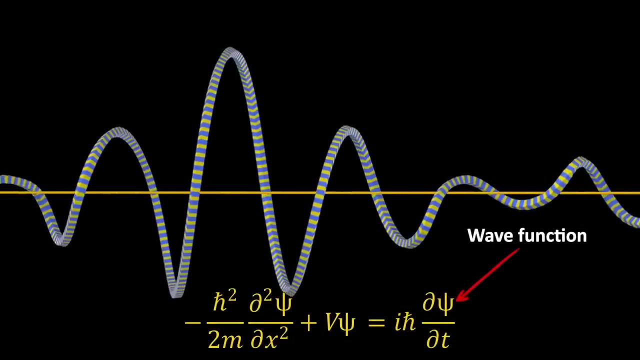 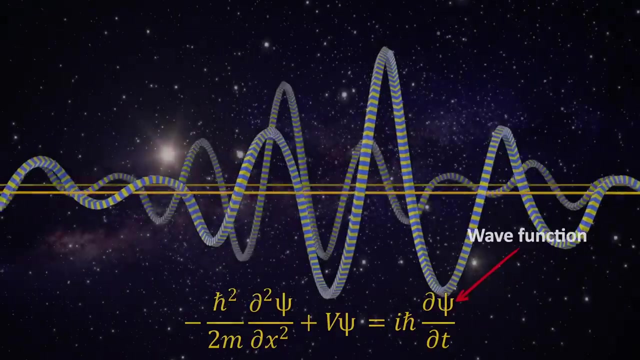 In classical mechanics, things are concrete. Objects have distinct positions and velocities. In quantum mechanics, objects have wave-like behavior. they are more specifically described by wave functions, which are abstract mathematical solutions to the Schrodinger equation. These waves aren't localized, but instead take up all of space. 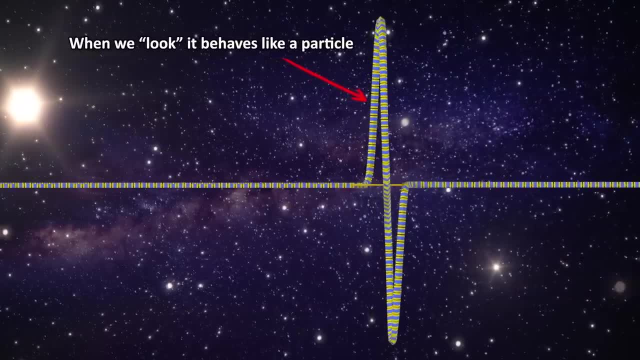 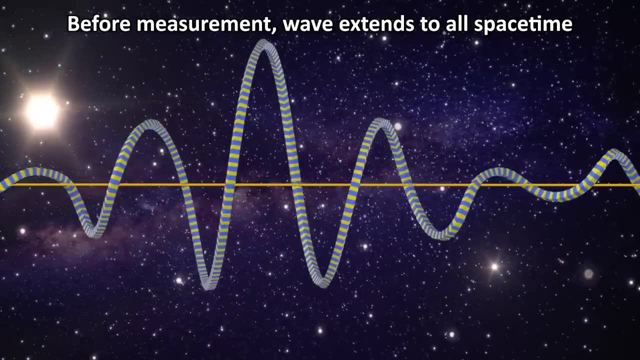 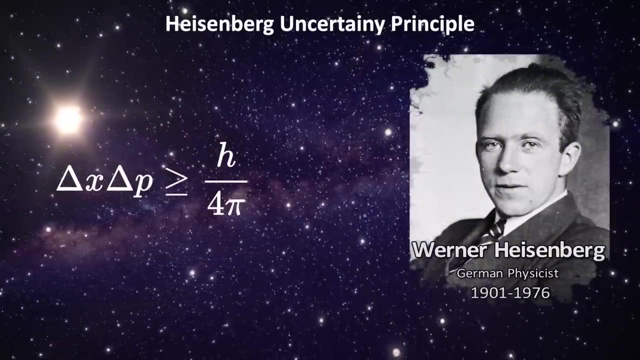 It isn't until you look for a particle that it becomes what appears to be a particle. Before that, the particle is a collection of probability waves that theoretically extend out to the entire universe. Now this has some pretty profound consequences. One is called the uncertainty principle, which states that you can never simultaneously know. 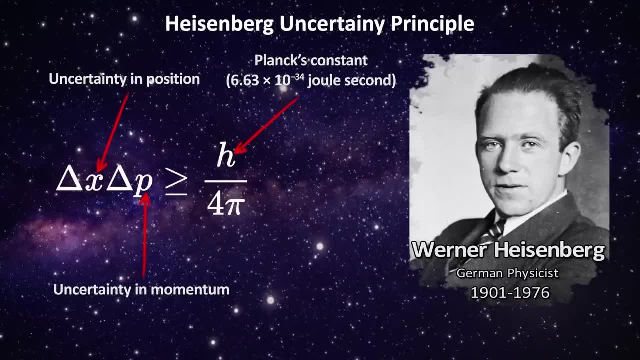 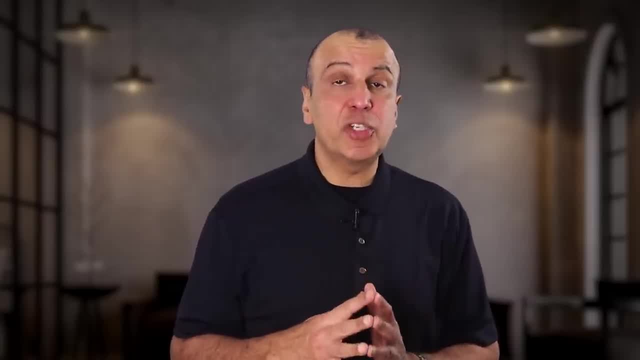 exactly where something is and how fast it is going. More precisely, we cannot know the position and momentum at the same time. This has to do with the probabilistic nature of quantum mechanics. Let's do an example to understand why this is the case. 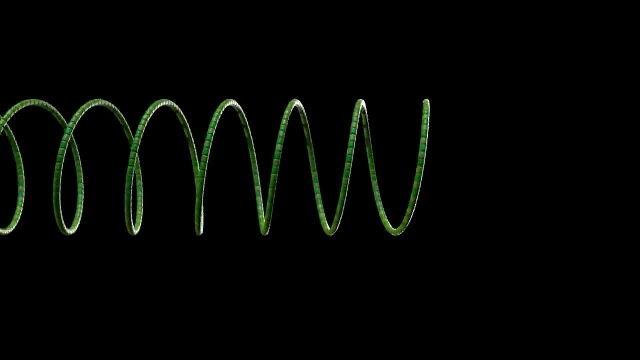 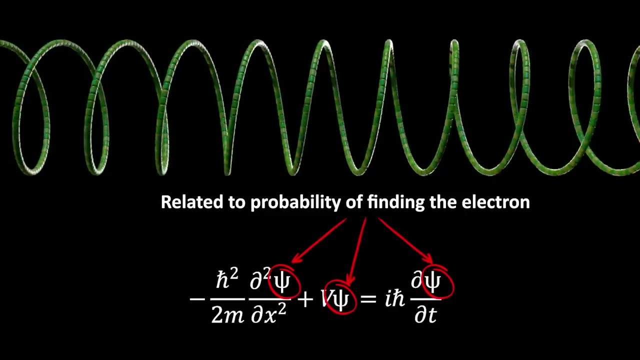 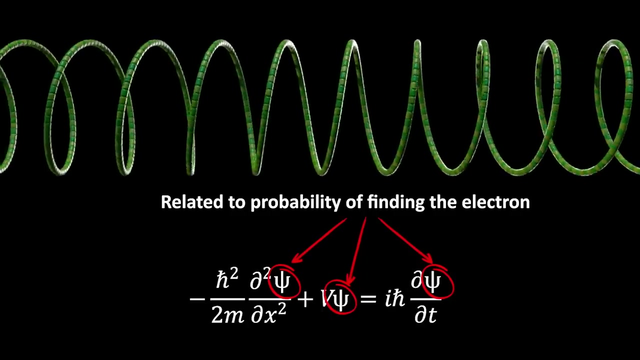 Where an electron is, because it's a wave. what we mean by wave is the wave function from the Schrodinger equation And this is related to the probability of finding the electron at any point in space. But a perfect sine wave for the electron spreads that probability throughout all of space. 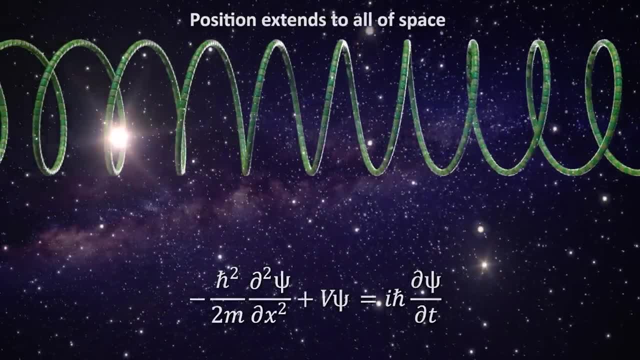 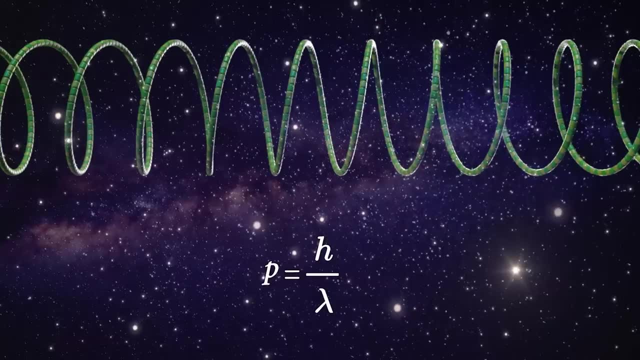 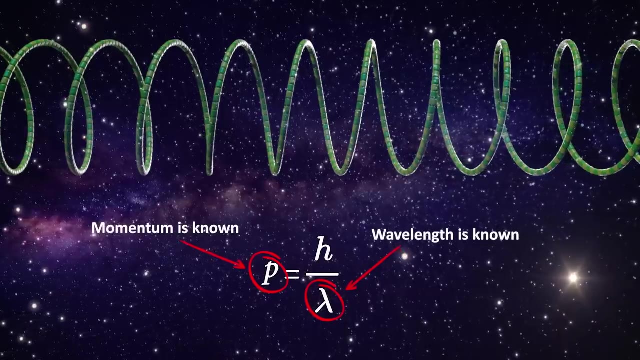 So the position of the electron is completely uncertain. But a perfect sine wave means we know it's the wavelength, so we would know its momentum, quite precisely because of the de Broglie relation, where momentum equals Planck constant over the wavelength. So in this case we have an infinite uncertainty in position, but no uncertainty in momentum. 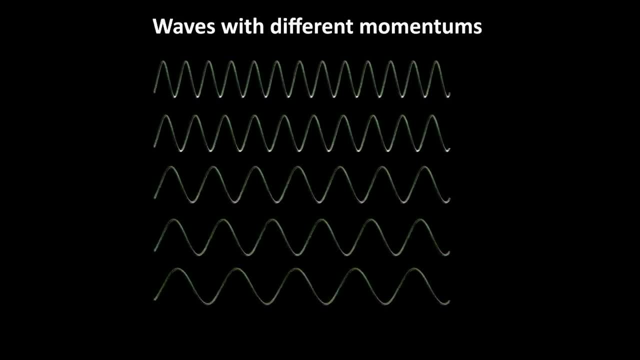 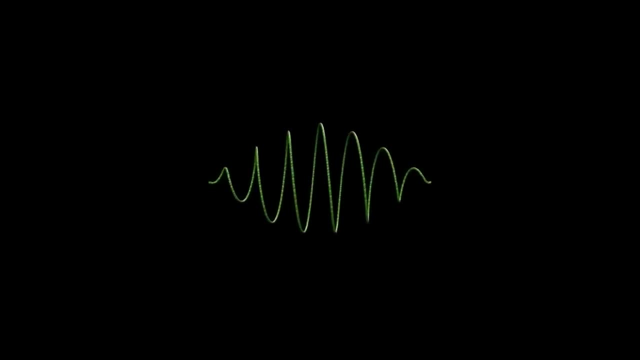 On the other hand, if we want to know the position of the electron precisely, we would need to add many waves of different wavelengths so that we can get an interference pattern such that we get a more localized wave. This localized wave would give us a more precise, precise, precise wave. 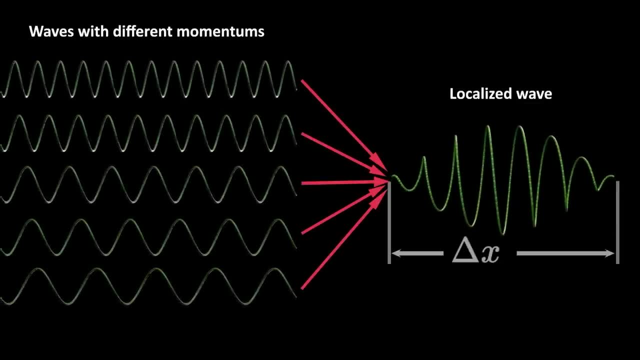 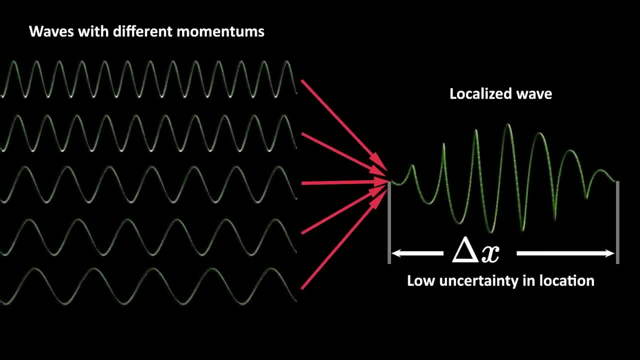 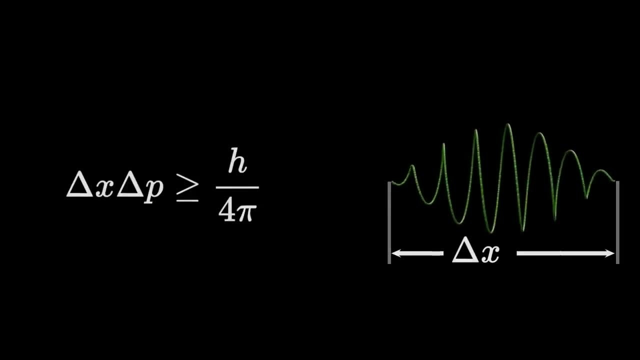 are of different wavelengths, have different momentums using the same de Broglie relation. So either we know the position very precisely or the momentum precisely, but not both. What's important to understand is that this is not a limit of our measuring equipment. 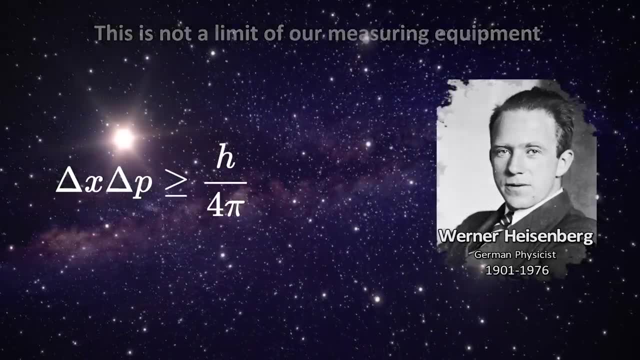 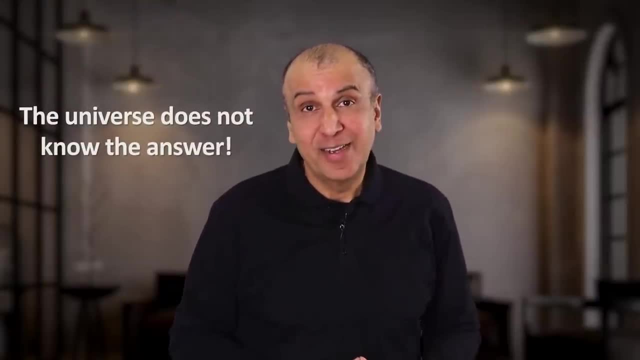 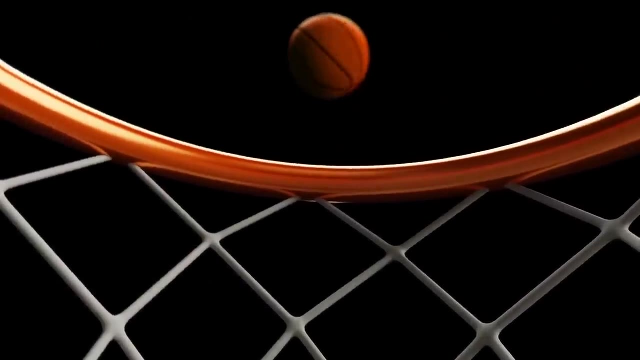 It's that exact answers to both the momentum and the position of a quantum object do not exist in the universe. at the same time, The universe itself doesn't know the answer. Now, this is hard to accept and goes completely against our everyday experience. So you have to ask: why don't we see this wave behavior in macro objects? 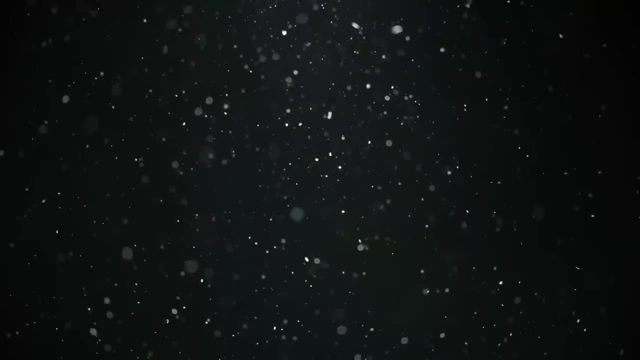 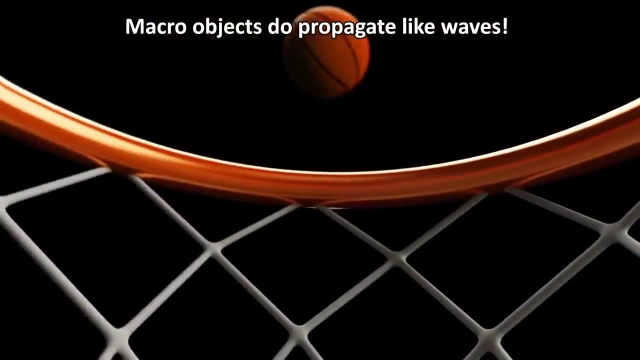 Like a basketball or tennis ball or even a tiny particle of dust. Well, I'll let you in on a little secret: Dust particles, tennis balls and basketballs do propagate as waves, Just like electrons. In fact, everything does. 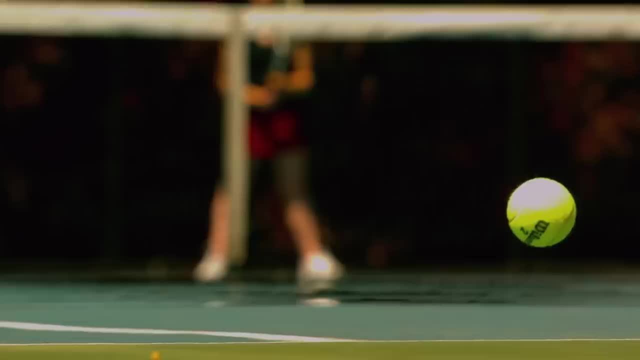 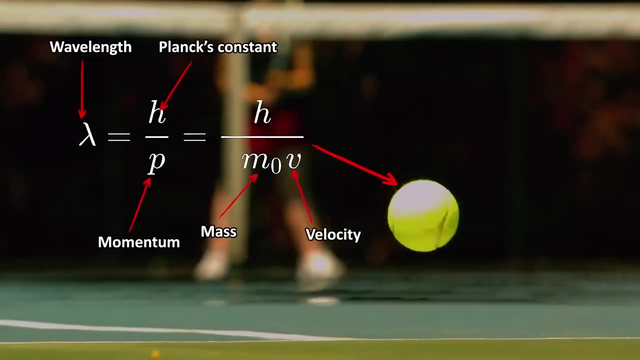 And their wavelengths can be calculated just like a photon or electrons. using de Broglie's formula. Wavelength equals Planck's constant divided by momentum, But for large objects the momentum is so much bigger than the Planck's constant that their wavelengths are an undetectable fraction of their physical size. 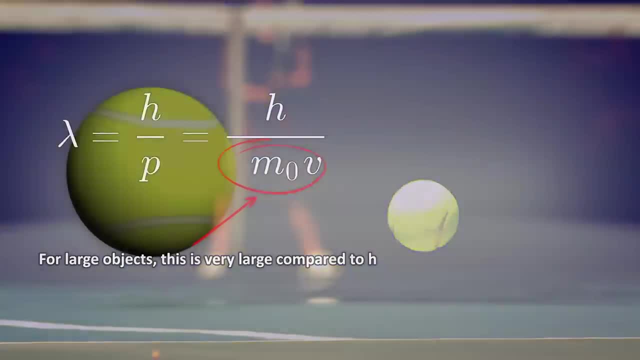 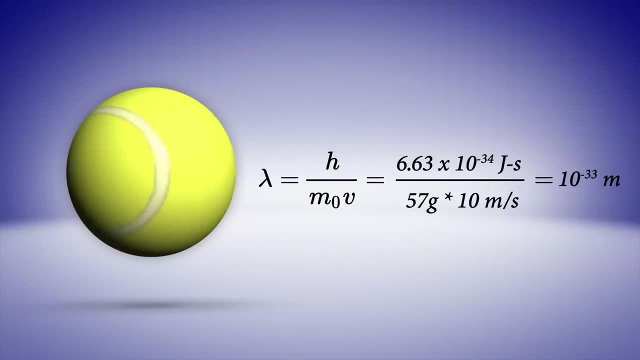 So we can never notice their quantum mechanical properties. For example, the wavelength of something the size of a tennis ball moving 10 meters per second Is 10 to the negative 33 meters. This is less than the width of a proton, So we would never notice it. 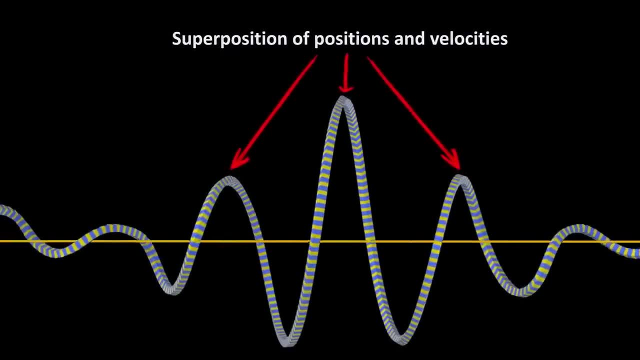 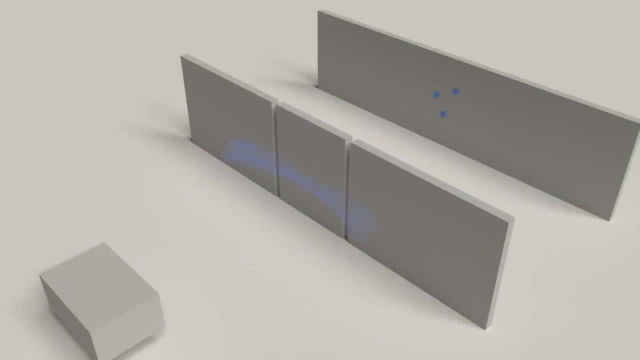 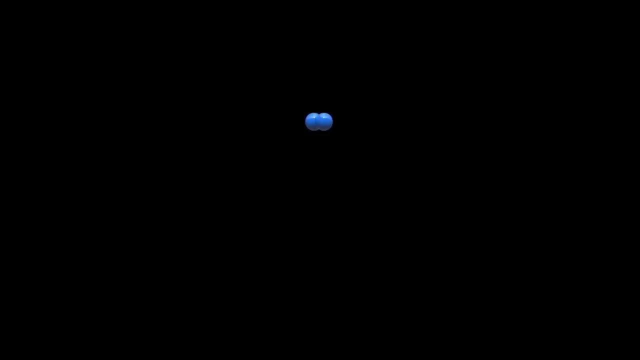 A second consequence of wave-like behavior is non-locality. A wave exists over multiple regions of space. This non-locality explains interference, but it also means that waves can add together to give complex interference patterns. So waves of multiple particles can add together to give a single wave function corresponding. 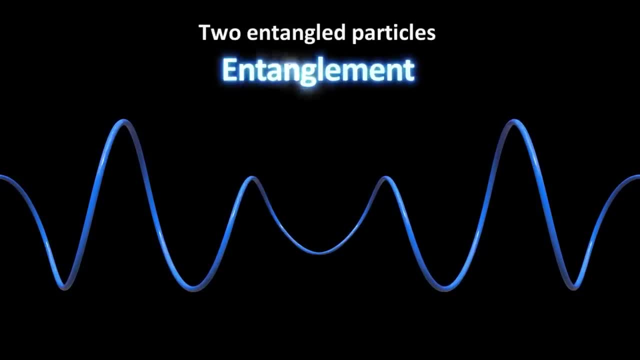 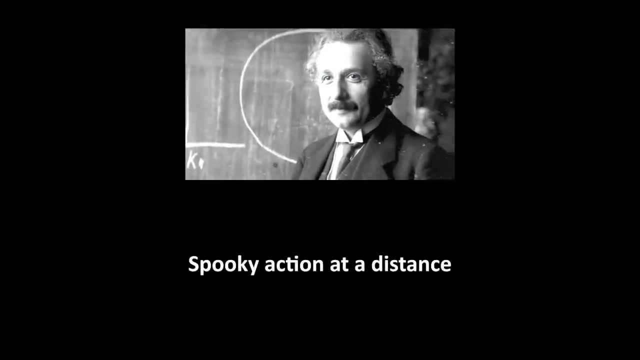 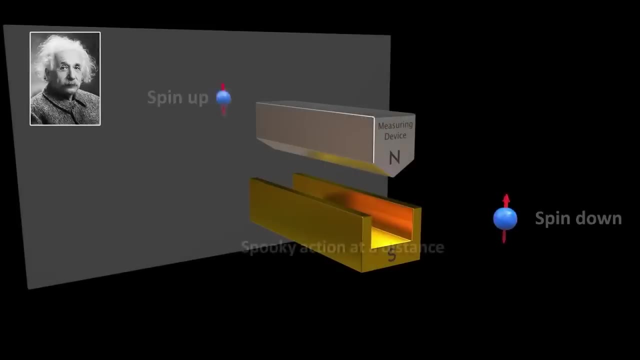 to multiple particles. This gives rise to a strange correlation between such particles in a phenomenon called entanglement. Einstein called this spooky action at a distance because it appears to indicate instant communication between distant objects at faster than the speed of light, which is forbidden by relativity. 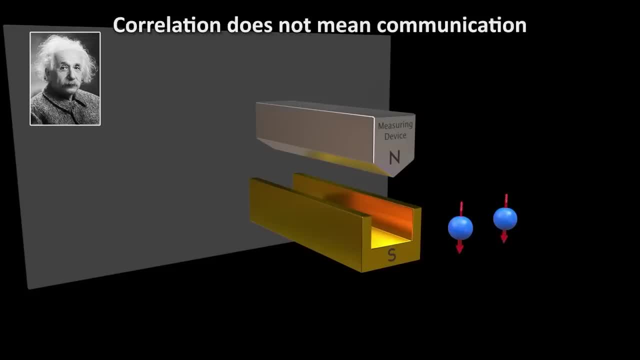 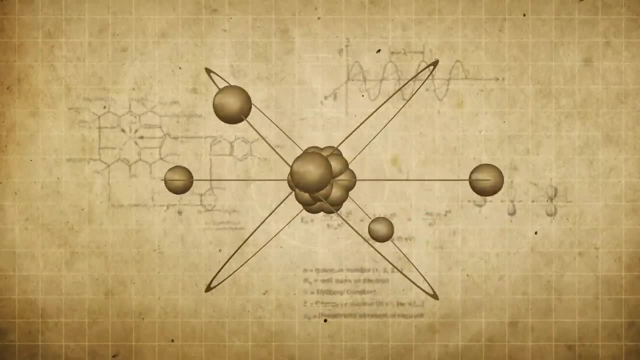 theory, But while two or more objects are correlated, no communication is actually happening. Correlation does not mean communication. The wave behavior is not the same. The wave behavior is not the same. The wave behavior of electrons also means that the concept of circular orbits of electrons 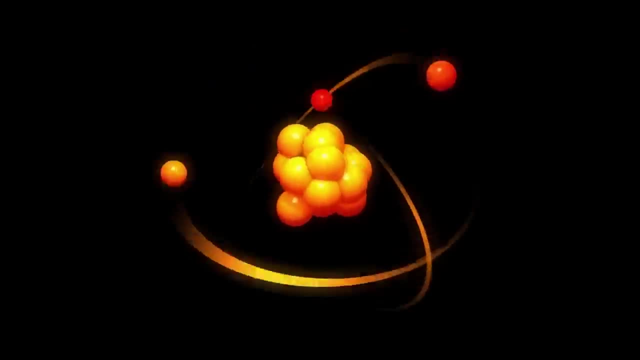 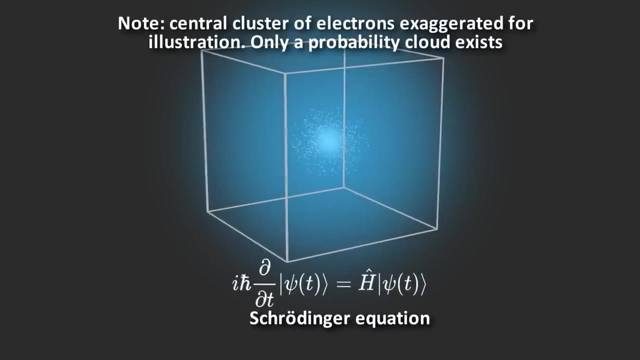 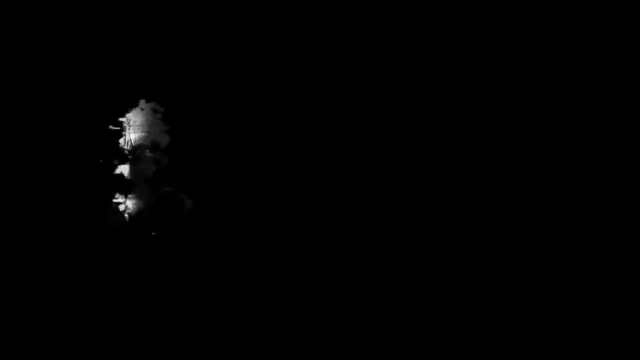 around the nucleus of atoms that you commonly see everywhere when an atom is depicted is wrong. A better picture is that they exist in a well-defined probability cloud around the nucleus that might look more like this: The main point is that the universe is quantized. 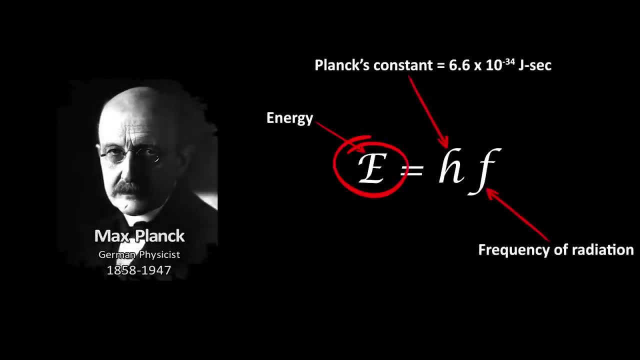 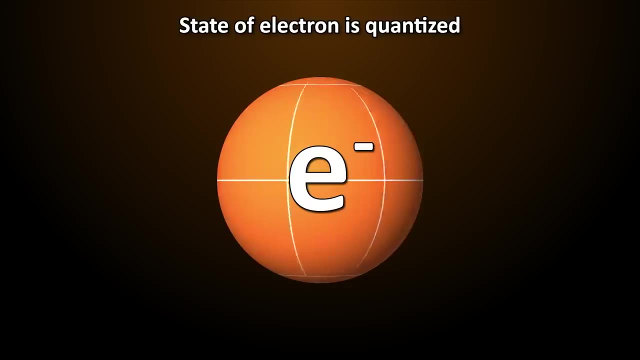 Familiar quantities such as energy, momentum, electric charge, mass And possibly even time and space are not continuous. they occur in discrete quantum units. So, for example, the state of an electron is quantized. By state I mean its energy, angular momentum and other properties. 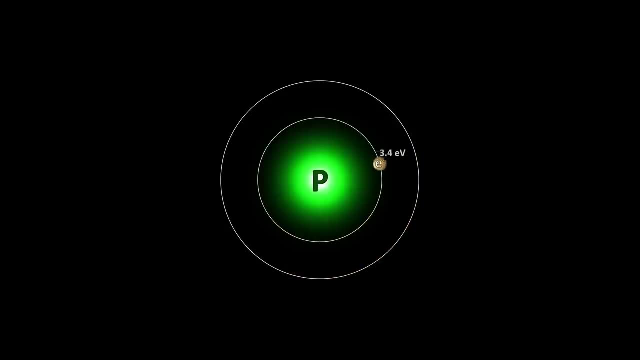 So an electron in a state of 3.4 eV of energy that moves to 13.6 eV of energy does not pass through any intervening energy values, It just disappears. It disappears from its old state and reappears in the new state. 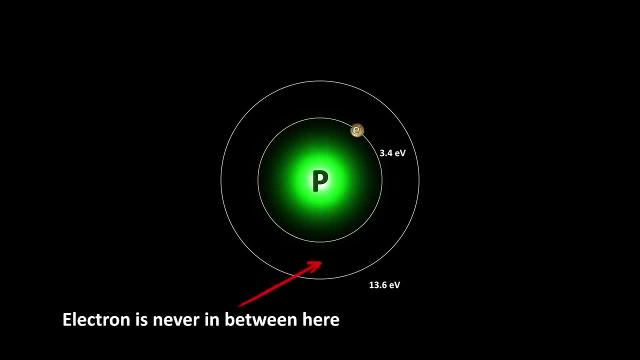 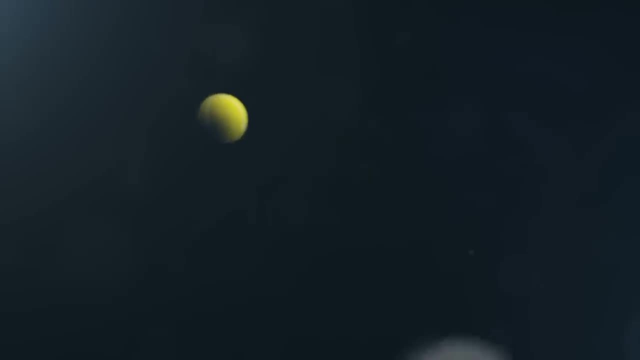 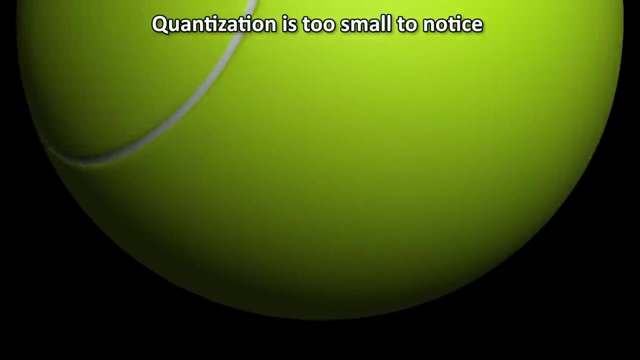 It never exists between these two states. This is how an electron moves from a lower energy shell of an atom to a higher energy shell. This quantization is not directly observable in our daily experience because the intervals between the units are too small for us to notice. 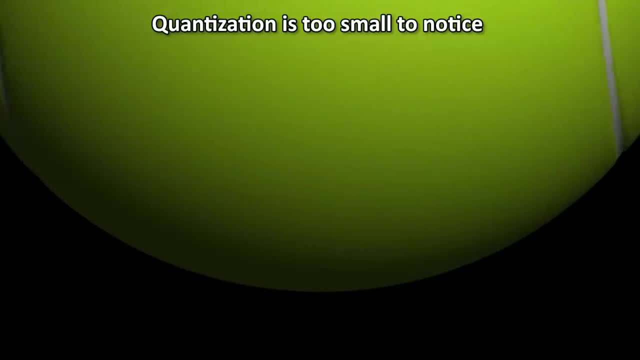 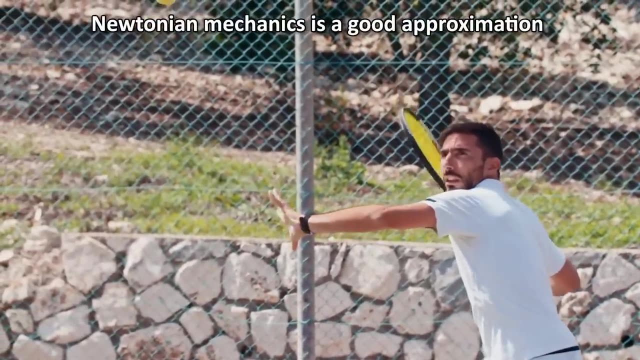 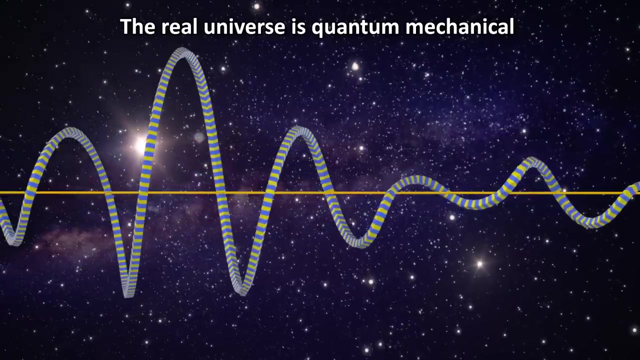 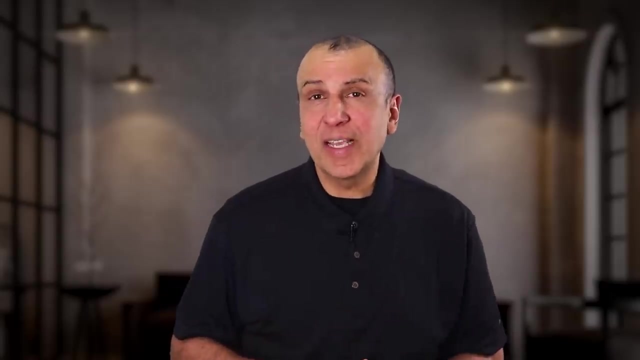 It isn't that quantum mechanics only exists at small scales. Quantum mechanics is all there is. It is everything. Newtonian mechanics, or the physics of our macro scales, just happens to be a good approximation of the underlying, more fundamental quantum mechanical universe. And if this makes you want to learn more about the fundamentals of quantum science, two of 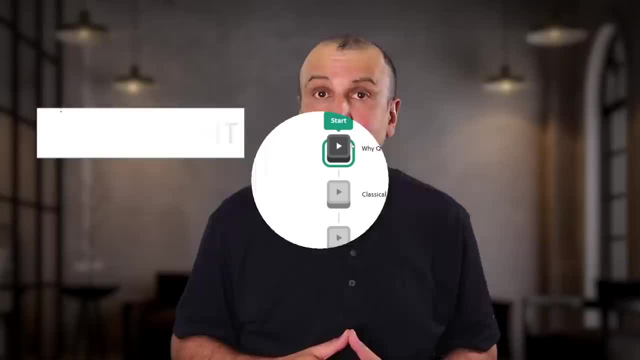 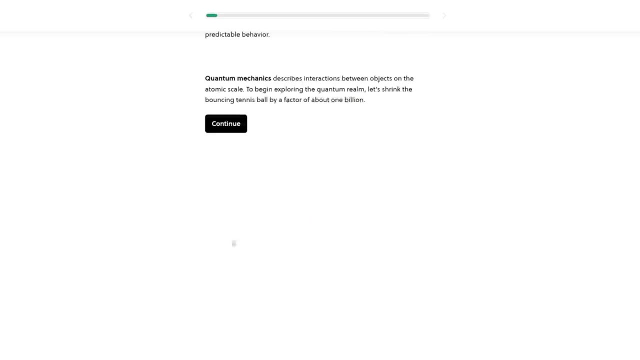 the best courses are available on Brilliantorg, today's sponsor. The first course I want you to look at is called Quantum Objects. It's an 18-lesson course that walks you through the fundamentals of quantum mechanics, from spin to quantum mechanics, From spin to the mathematical foundations, to Schrodinger's equation. it will give 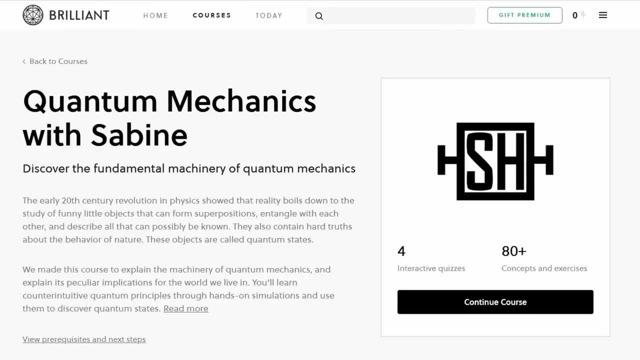 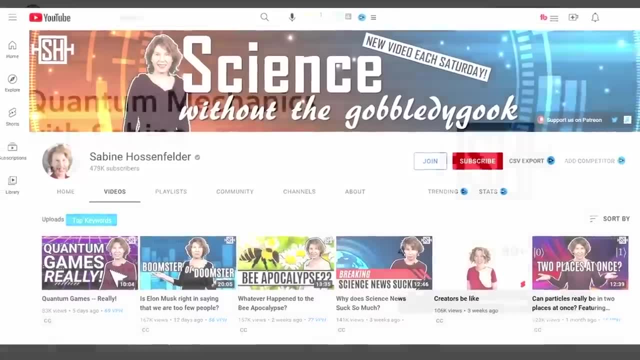 you the background you need for further study. The second exceptional course is a new one called Quantum Mechanics with Sabina, created with the collaboration of physicist and fellow YouTuber, Sabina Hassenfelder. She is a friend of mine and does a great job teaching about some of the counter-intuitive. 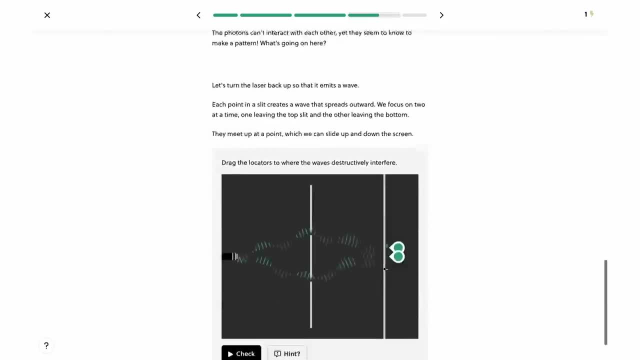 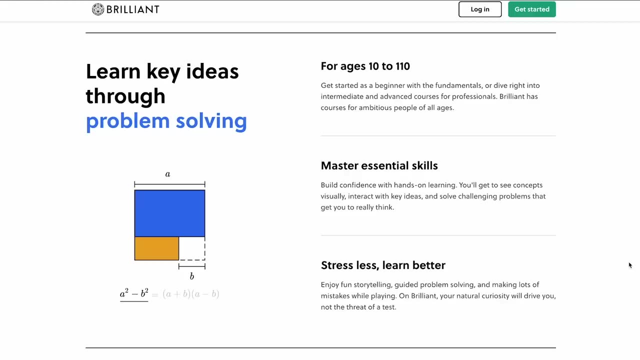 aspects of quantum mechanics, which will start to make better sense as you go through the course. The unique thing about these brilliant courses is that they use hands-on simulations, interactive quizzes and visual demonstrations. In my opinion, it's a better and more fun way to learn normally difficult subjects. 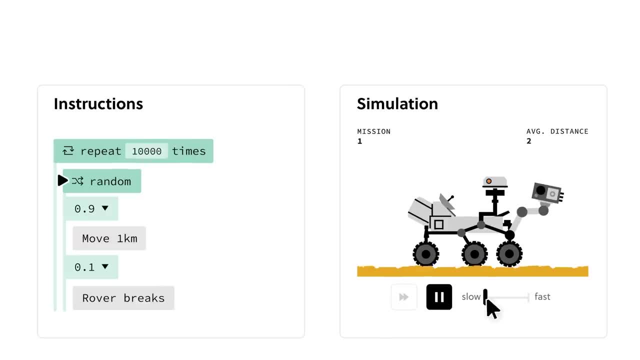 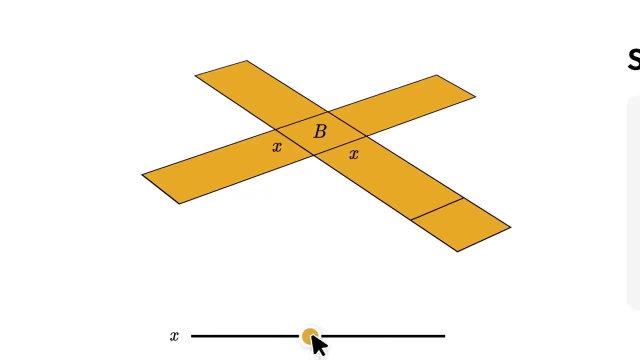 Brilliant has something for everyone, with thousands of lessons over a variety of STEM courses, with new content added each month. With as little as 30 minutes a day, Brilliant can help you develop your STEM skills and become a better thinker. Brilliant has a special offer for Arvind Ashfier's right now. 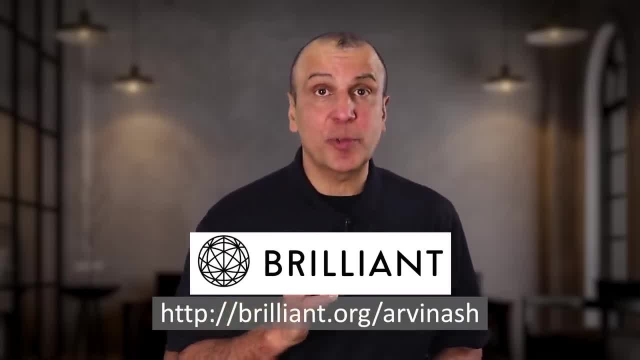 Get started for free for a full 30 days by clicking the link in the description. The first 200 people will even get 20% off the course. Brilliant has a special offer for Arvind Ashfier's right now. Get started for free for a full 30 days by clicking the link in the description.